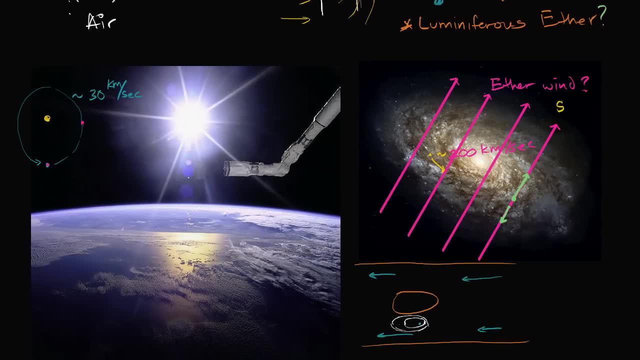 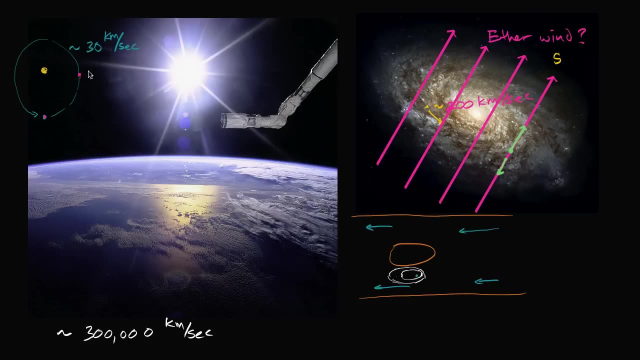 or why did they feel confident that there was a relative velocity? Well, we talked about that in the last video. The Earth is spinning, and then it's orbiting around the sun at a nice clip, and then the whole solar system is orbiting around the center of the galaxy at a nice clip. 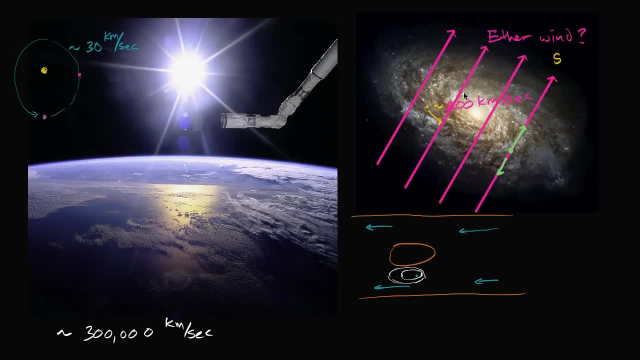 The galaxy itself might be moving. So if you have some absolute frame of reference that's defined by the ether, well, we are going to be moving relative to it. And if you said, okay, if we're moving relative to it, well, maybe you just measure the speed of light. 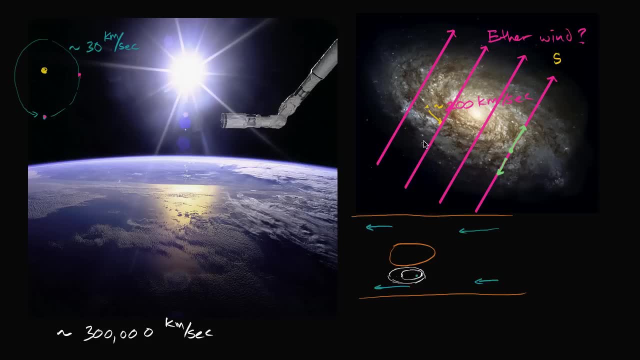 in different directions and see whether the speed of light is faster or slower in a certain direction, and then that might help you to identify well one. validate that the ether exists, but also think about what our velocity is relative to the ether. 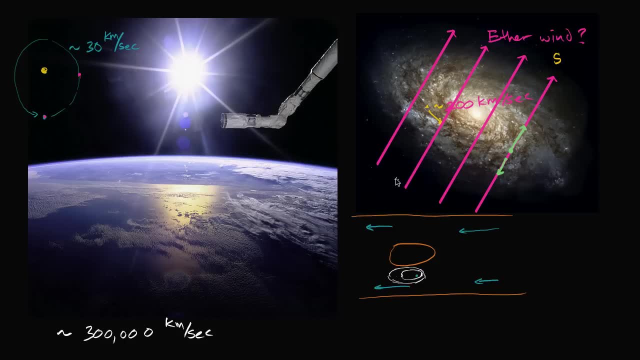 relative to that absolute frame of reference. But the problem in the 19th century is that we did not have any precise way of actually measuring or a precise enough way of measuring the speed of light where we could detect the relative difference due to the light going for or against. 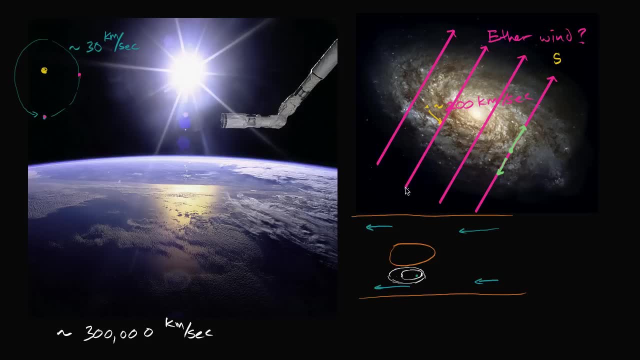 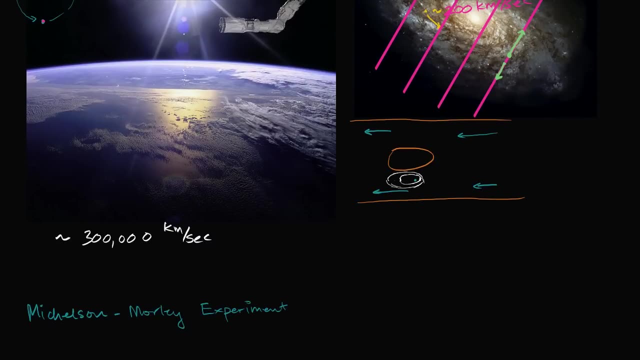 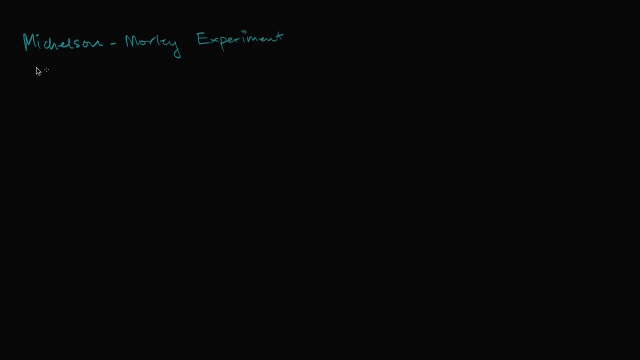 or into or away from the actual direction of the ether wind. And so the experiment that is usually cited with first kind of breaking things open and starting to really make a dent in this whole idea of a luminiferous ether is the Michelson-Morley experiment. 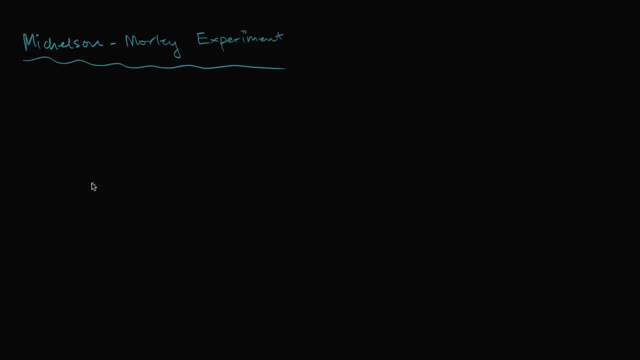 Michelson-Morley experiment. They recognize. okay, we can't measure the speed of light with enough precision to detect has it gotten slowed down by the ether wind or sped up by the ether wind. but what we could do, and this is what Michelson 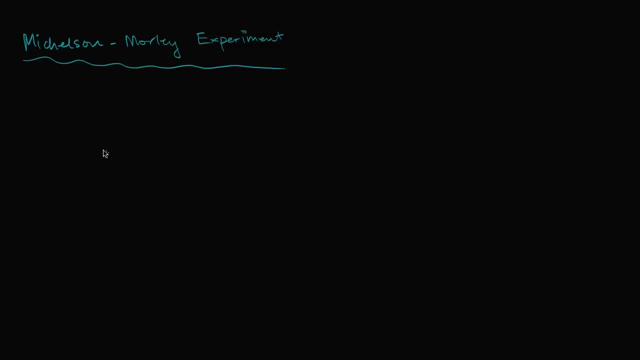 and Morley did do, and I'm gonna do an oversimplification of the experiment- And they said: okay, you have a light source, You have a light source right over here, So you have a light source And so that's going to send light in this direction. 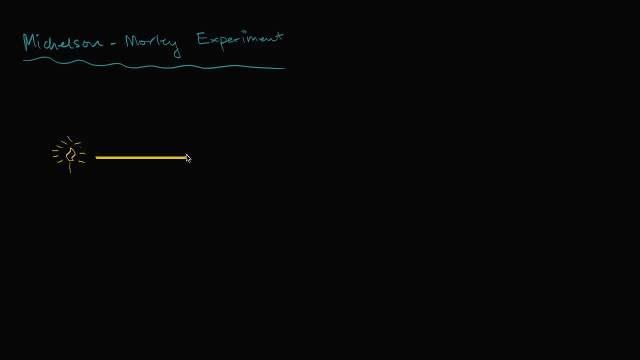 It's going to send light just like that, And what you do is you have a half-silvered mirror that allows half the light to pass directly through it and half of it to be reflected. So let's put a half-silvered mirror. 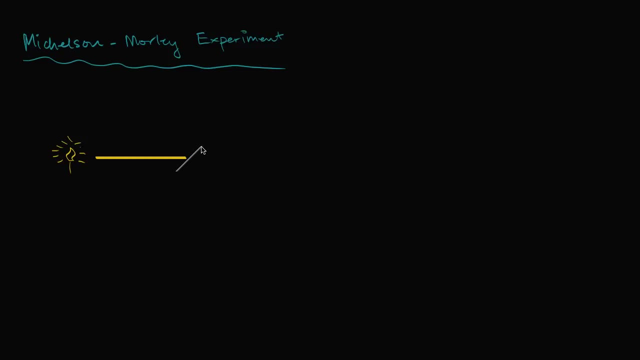 right over here. So there's a half-silvered mirror And so half of this light will bounce off like this. This is just a simplification of it. Let me do it a little neater than that. So half will bounce off like that. 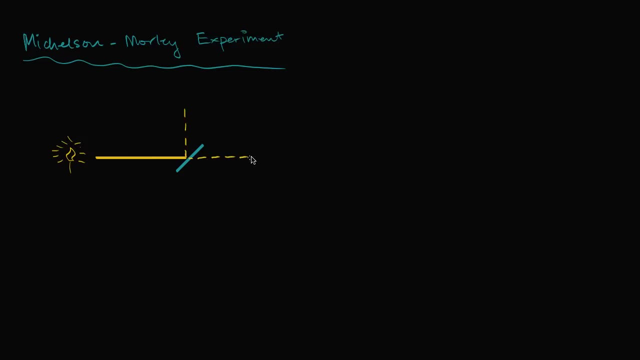 And then the other half will be able to go through. it Will be able to go through it. It's a half-silvered mirror And then we make each of those light rays. we've essentially taken our original light ray and split it into two. 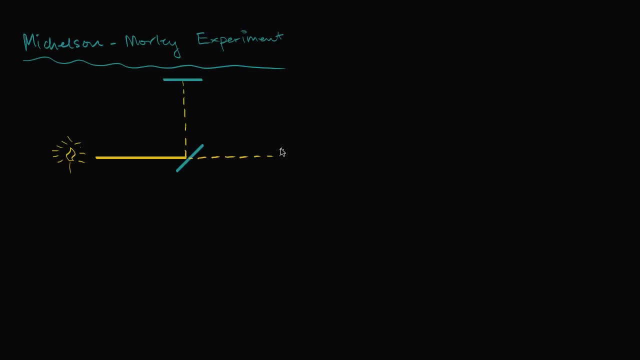 We'll then bounce those off mirrors. Bounce those off mirrors that are equidistant, And there are some adjustments when you actually have to factor in everything, But just as a simple notion, these things are just now going to bounce back. So this one is now going to bounce back. 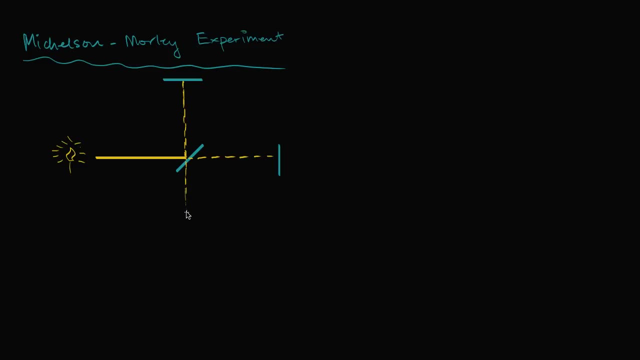 It's half-silvered, It can go through, or part of it can go through, that mirror. So that's that ray, And then this one is going to bounce back, This one's going to bounce back, And part of it is going to bounce back. 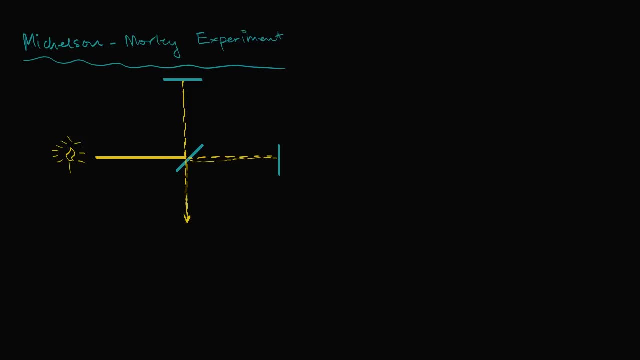 This one is going to bounce into this direction, And then you can detect what you see. You can detect what you see. So this right over here is a detector. And you might be saying, okay, Sal, well, what's the big deal? 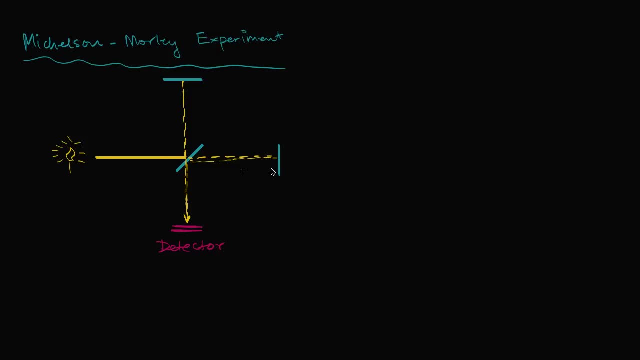 You've taken a light source, You've bounced, you've split the light rays, You've put them back together, You've bounced them around a little bit. But think about if there was a luminiferous ether, these light waves that are going in orthogonal directions. 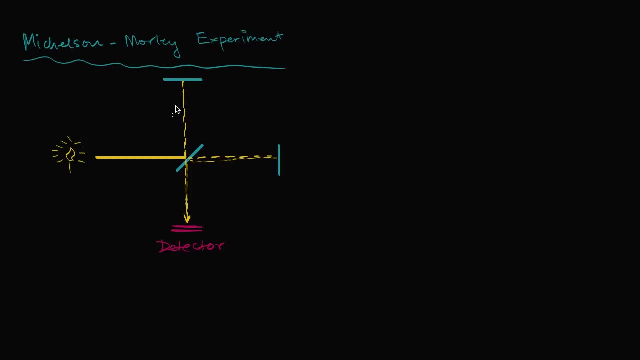 will be going at different velocities. Let's say, if that luminiferous ether was, if the ether wind was doing something like, let me see if the ether wind were in this direction. if the ether wind were in that direction when the light wave is going that way. 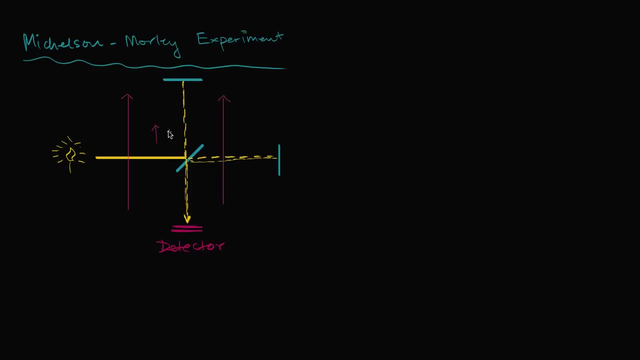 it should be going faster, And when the light wave is coming back, it should be going slower. And so what Michelson and Morley did is okay, let's assume. let's adjust our apparatus right over here, So when these two light rays bounce off, 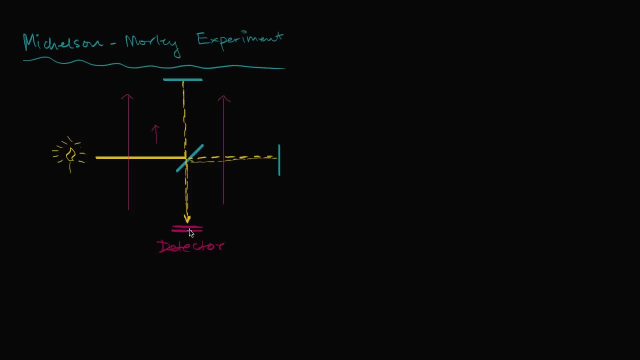 and then come back together. if there were no ether, you would have some basic interference pattern. So what do I mean by interference pattern? Well, let's say that you have maybe this one bouncing from up here. Let me do that in a different color. 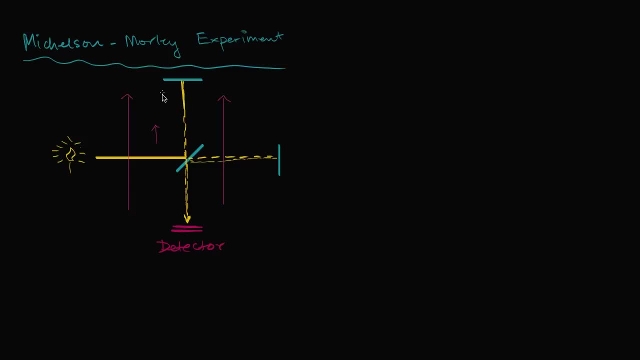 So the one bouncing from, the one bouncing from up here, let's say that that is looks like this. I'll just draw it as a longitudinal wave, just like this- Best a hand-drawn longitudinal wave. And then the one coming from the other direction. 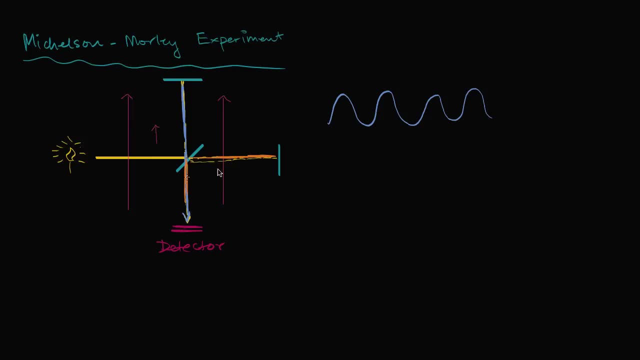 the one that bounces here and then comes back like this is another longitudinal wave like this, And when they overlap they are going to interfere with each other, either constructively interfere or destructively interfere. So you could have something like. you could have something like this: 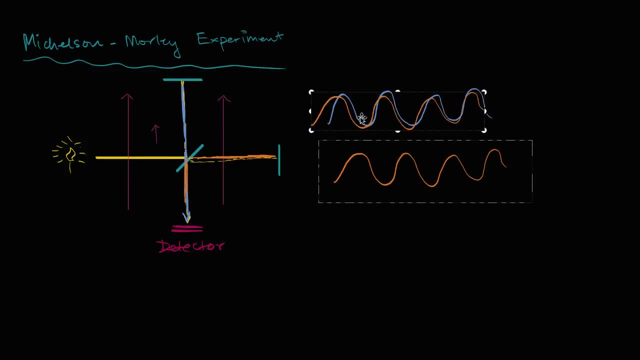 So let me copy and then let me paste it. So, depending on how far, how fast each of these traveled, you're gonna have different levels of interference And you would have a difference depending on the orientation, depending on what the actual ether wind is doing. 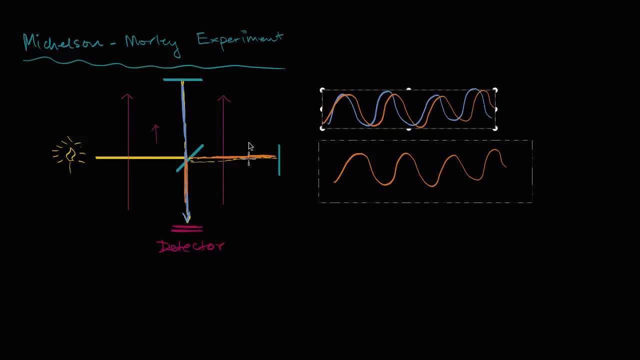 But what Mickelson and Morley observed is that no matter how they oriented this apparatus- and they did it at different times of the year, and they rotated around, and they rotated in the vertical direction, in the horizontal direction, no matter what they did- 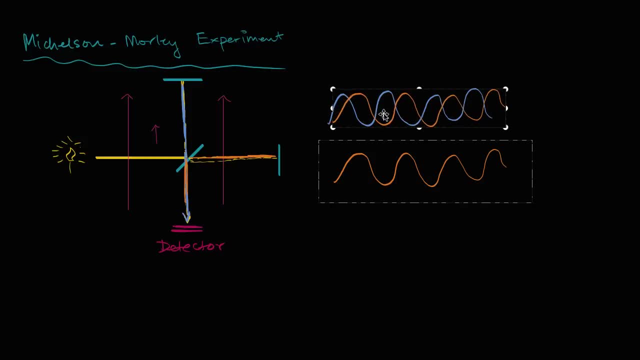 they always got the same interference pattern. The interference pattern did not change And because the interference pattern did not change, it implied that, well, maybe this ether isn't really having an effect on slowing down or speeding up the light waves. So this was is often called. 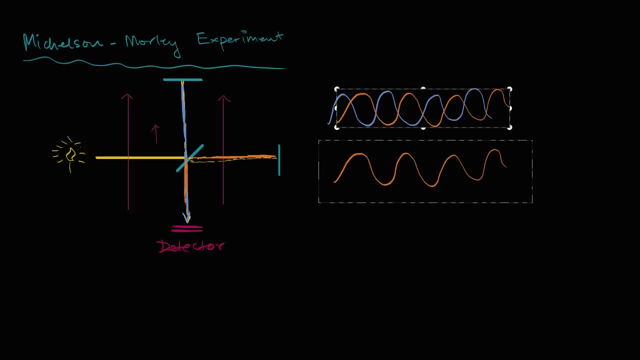 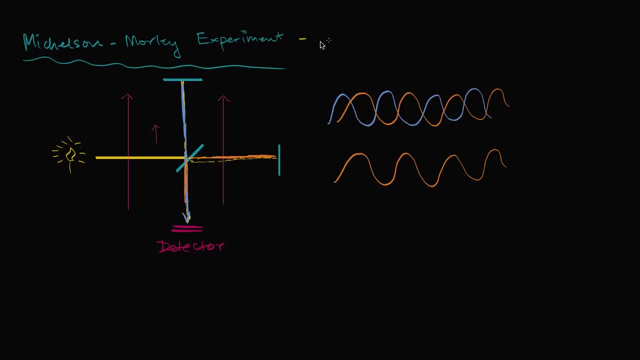 one of the most famous failed experiments in physics. So let me write this down. What's powerful about it is that it was a failed experiment. Let me get my pen down. Let me get my pen tool out. It was a failed, failed experiment. 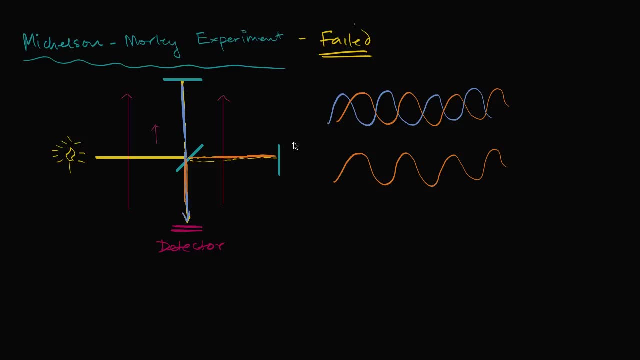 but it made people start to question: well, maybe there isn't an ether, a luminiferous ether, Maybe light just somehow travels through the vacuum, Maybe there is not this absolute frame of reference, this defined by the luminiferous ether?